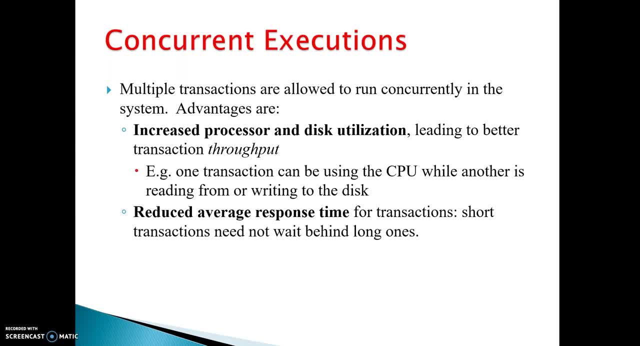 It indicate like multiple transactions are allowed to run concurrently in the system. So if you can do like this, what is the advantage? So basically, increase the processor and disk utilization So it leads the better transaction throughput. Here particularly, we would like to mention 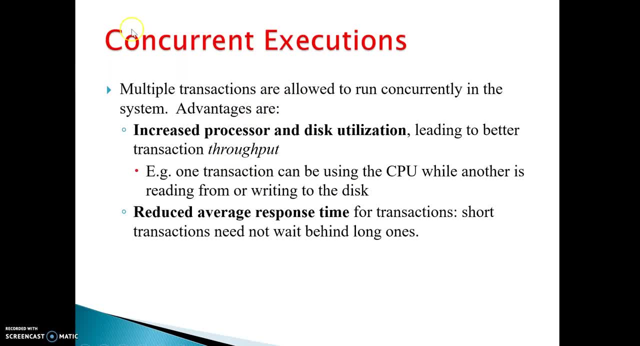 one important keyword is throughput. It indicates number of transactions performed in a unit time. indicate throughput, So concurrently executed number of transactions. it leads to increase its throughput. One transaction can be using the CPU while another is reading from or writing to the disk. 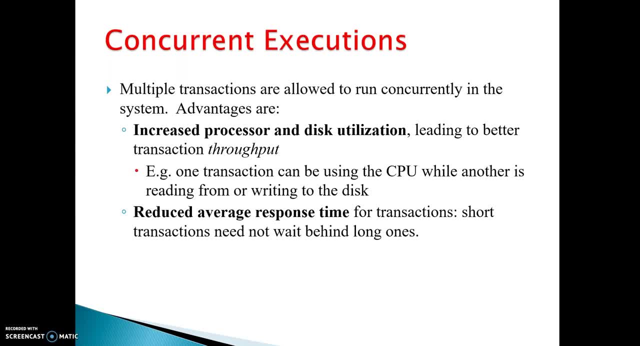 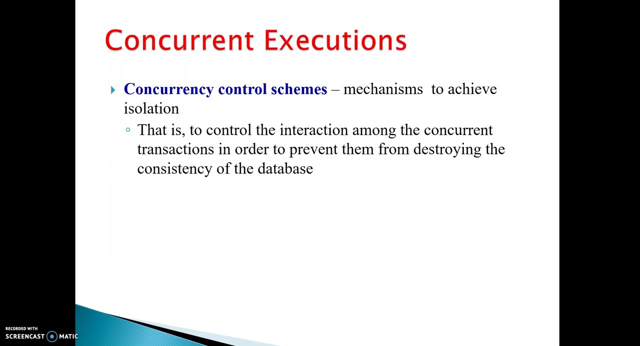 So another advantage with this concurrent execution is reduced average response time for a transaction. So it means the short transactions need not wait beyond long ones. So because of these two reasons, we normally prefer to execute transactions concurrently. If you can do like that, it means that concurrency- the transactions are going to be executed. 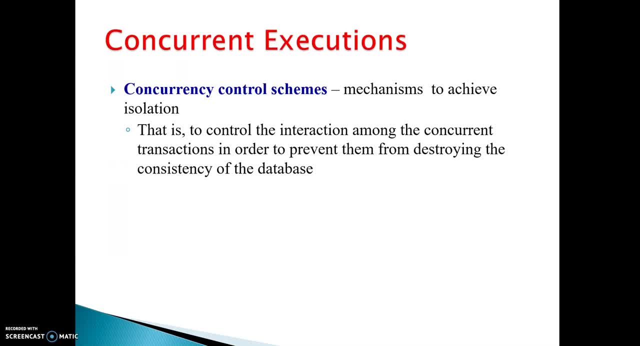 concurrently. we need to manage one mechanism, how we use it, to control these entire things, otherwise it leads to some inconsistency and other kind of issues that well come into a picture. Toamos can schemes through the isolation. This is to control the interaction among the concurrent. 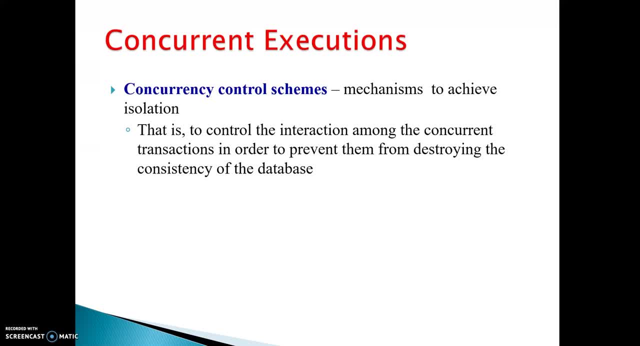 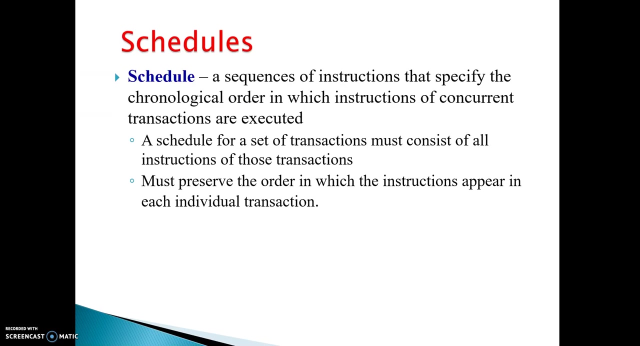 transactions in order to prevent them from destroying the consistency of the database. So basic aim of the database is to maintain its consistency, But whenever it is going to be executed concurrently it needs to be performing some type of control mechanisms. So in this, first we need to look at make transactions into schedules. So that is the 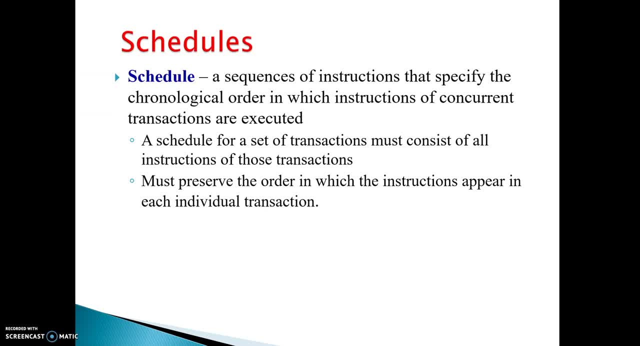 one of the important point here would like to mention schedules. It is a schedule. What exactly is a schedule? It is a sequence of instructions that specify the chronological order in which instructions of the concurrent transactions are executed. Then our more number of transactions are going to be executed in a chronological order. 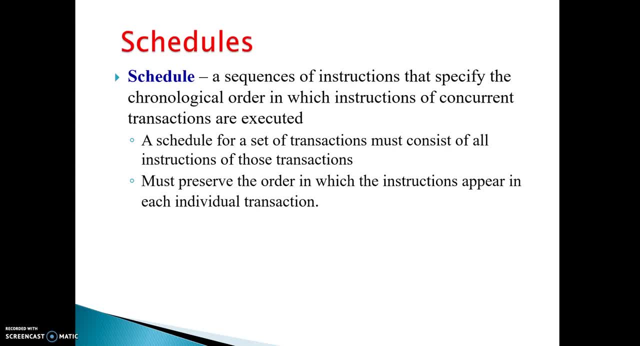 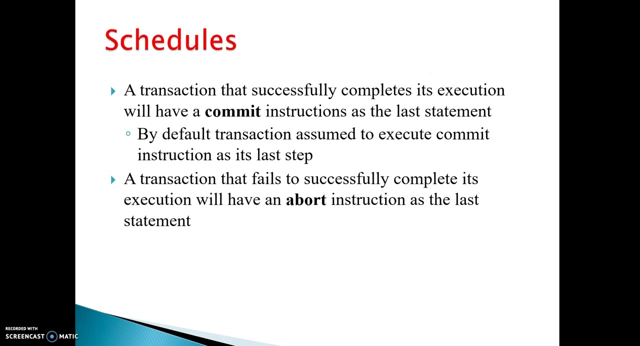 A schedule for a set of transactions must consist of all instructions of those transactions. So according to this, scheduling must preserve the order in which the instructions appear in each individual transaction. The order of the execution of transaction most of the time is very important aspect. So a transaction that successfully completes its execution. 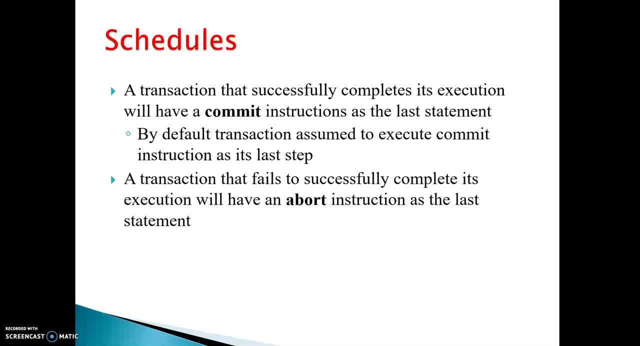 will have a commit instruction As the last statement. By default transaction assumed to be executed, commit instructions as it last step. So once it leads to the commit, it indicated that your entire transaction performed properly. A transaction that fails to successfully complete its execution will. 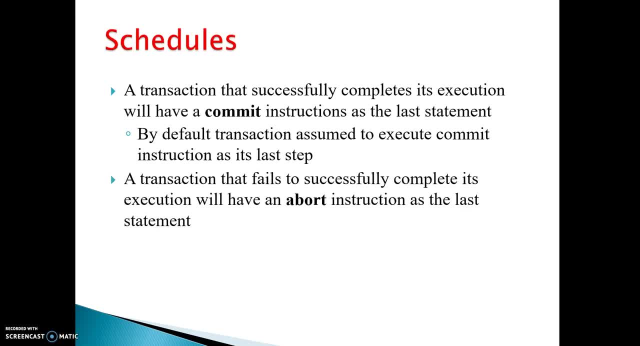 have an abort state, The instruction has the last statement. So then here important aspect about in the earlier slide, in the earlier presentation we discussed there are five states. one among about is one state where the transaction aborted because it has not happening properly. So let us see how the scheduling is happening. 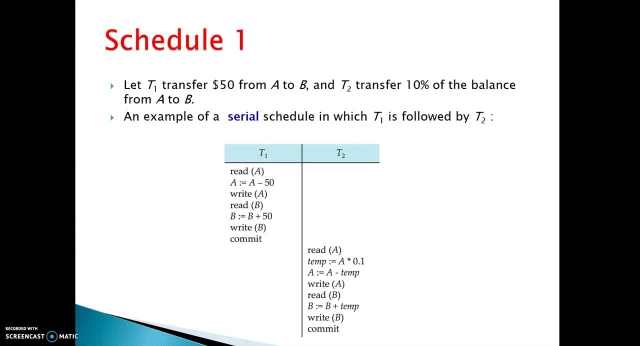 and planning in this. Let us use the same example in the earlier presentation. Let there is a transaction D19.. D1 and D2 here. in this case, Let us D1 performs transfer $50 from A to B And transaction D2 transfer 10% of the balance from A to B. Look at this schedule, An example serially: 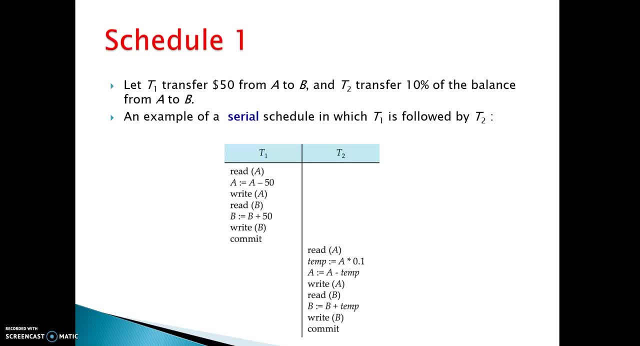 the transaction one and two executed. Look at here. Keep in mind ecвон T1. transaction T1: execute first In this transaction T1 transfer $50.. deducted from A, write A and add this $50 to B account and at the end commit. 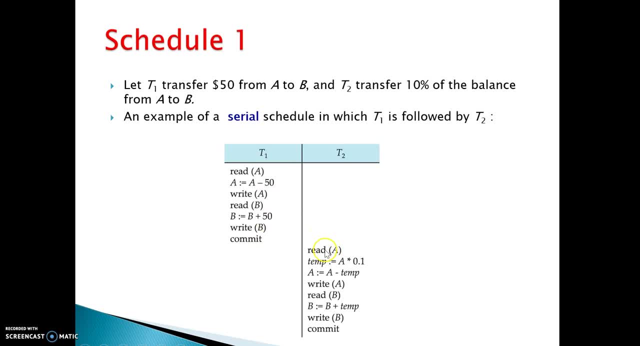 transaction 1 to B: complete Transaction two started. So when Transaction two starts According to the transaction 10%, transaction 2 is completed. So when transaction two starts according to transaction two, 10%, transaction 1 is completed and transaction two started. 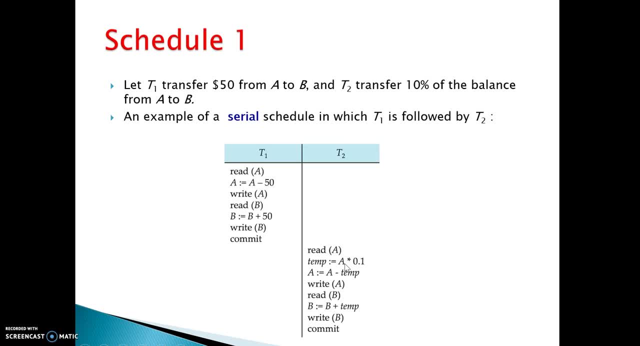 of amount from the A account will be stored into the temporary variable and deducted from this temporary variable from the account A and save it. And now this 10% amount will be added to the B account. The serial is the transaction as executed. It indicates serial means one after another. T1 is completed, then T2. 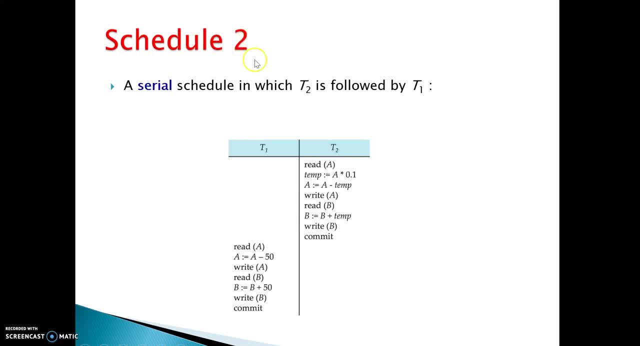 enters. Look at another schedule here, a serial schedule, in which T2 is followed by T1.. First look at transaction: T2 executed, then followed by T1. See here: in this case the final value has been transferred from transaction, I mean from the account. A to B has been bit changed. 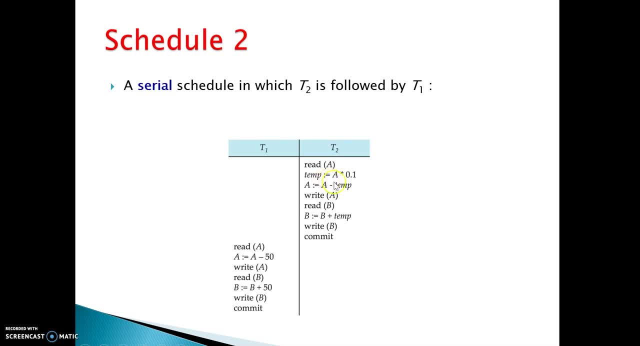 Here, in this case, look at 10%, initially after deducting. according to the earlier schedule, 1 deducted $50 from the account here, then after find the 10%, but transaction 2 executes first here. in this case, first 10% is stored in the temporary variable. 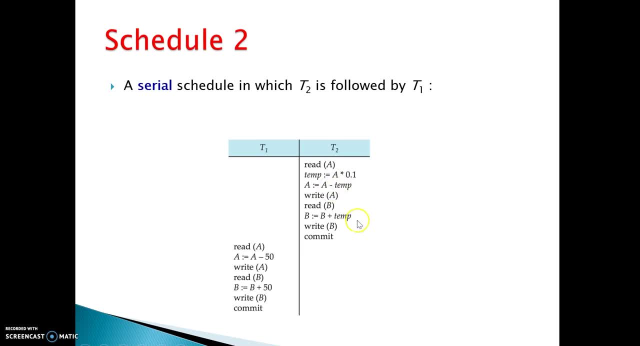 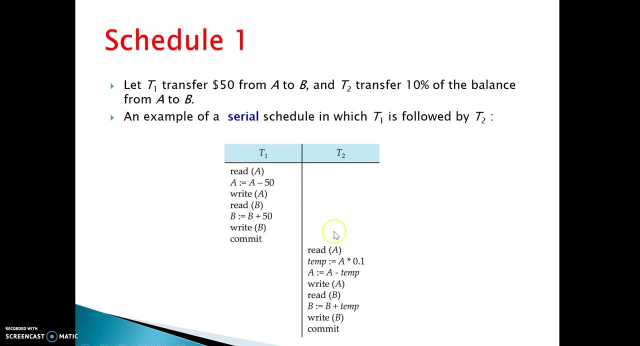 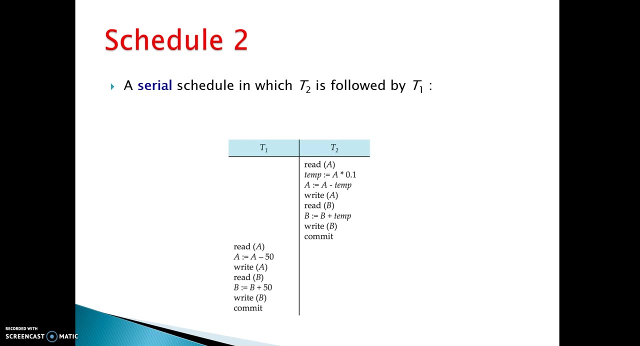 and subtracted from the account A and B, added this temporary variable 10% into B account. this result and schedule 1 results might be different. values can be transferred from account A to B once the serial serial scheduling has been changed. so look at the results of schedule 1. look at the result of schedule. 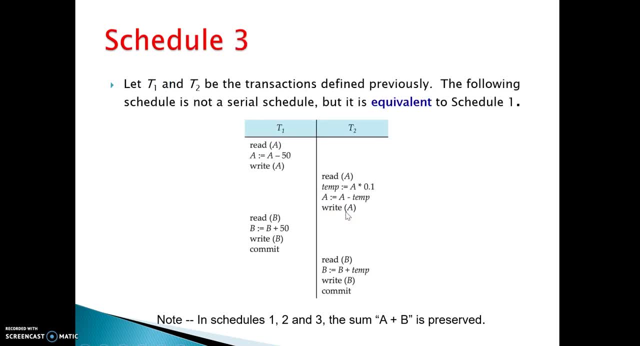 2 might be different. look at into the schedule 3. in this T 1 and T to be transactions defined previously. in this T 1 and T to be transactions defined previously. The schedule is not in a serial schedule but it is equaling to schedule 1.. 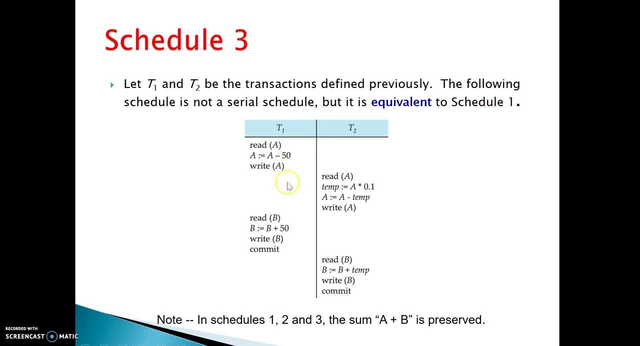 But happening. look at here in the transaction T1, first 3 instructions executed, then come to the T2, and first 3, 4 instructions executed, T2, and switch over to the T1.. So here the transaction T1 and T2 executing simultaneously but switch over the execution.